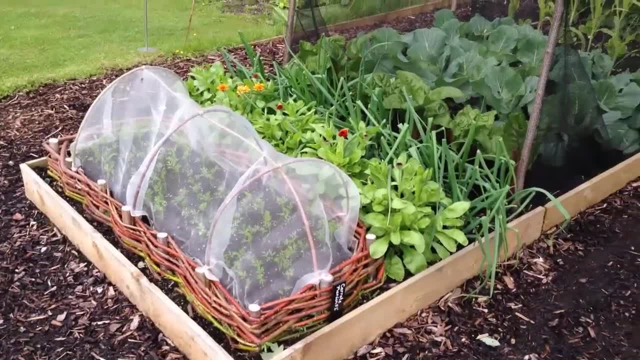 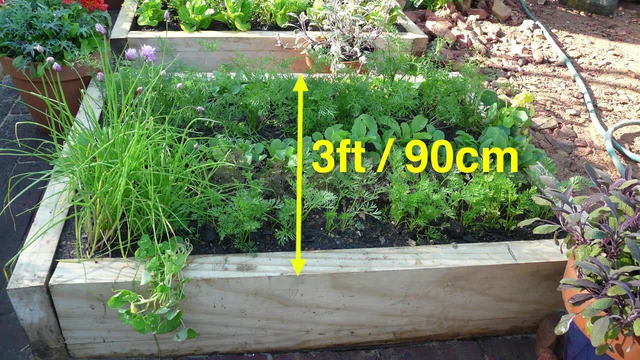 or a hard surface such as a concrete yard. Fill the beds with nutrient-rich potting soil and compost. Beds shouldn't be any wider than 3 foot across, so the children can easily reach the middle from the sides. Woodchips are a good way to start your garden. 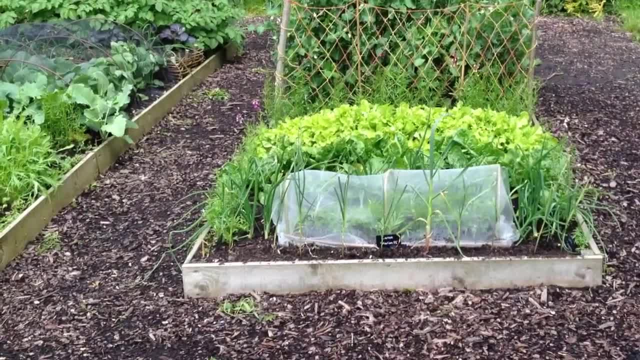 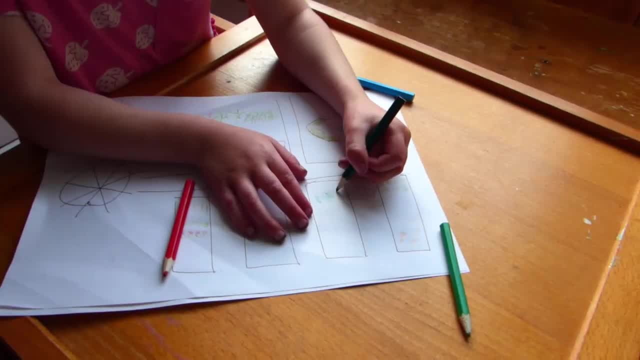 Woodchips are a good way to start your garden, and they're a good choice for the paths in between, as they're relatively clean and soft. If your garden is going to be a little more than a few raised beds, then why not get the kids involved in the design process? 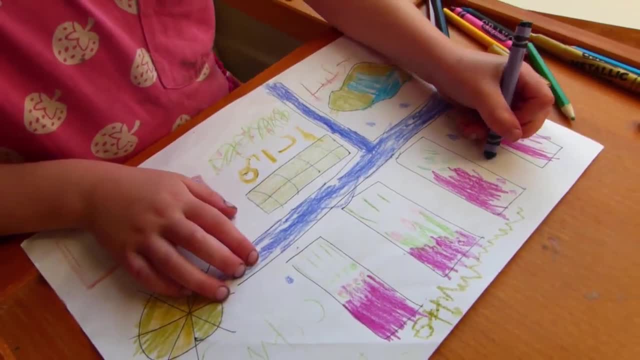 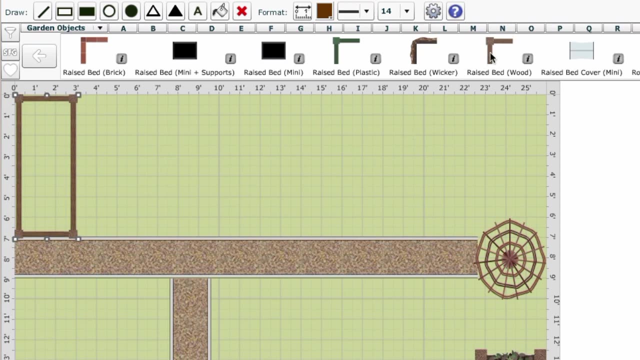 Ask them to make sketches or put together a mood board of what they'd like to see. They could even make their own design on a computer. Our online garden planner is child's play to use. Drop in garden objects such as paths, raised beds, compost bins and bean wigrams. 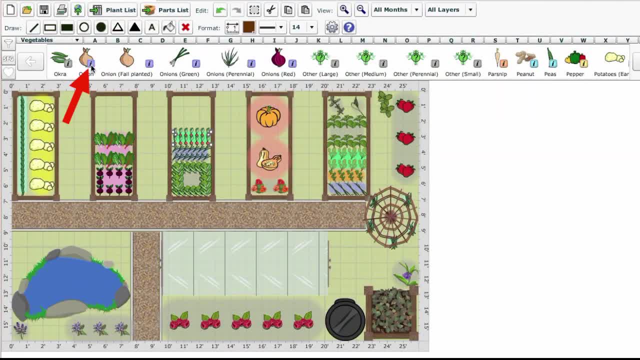 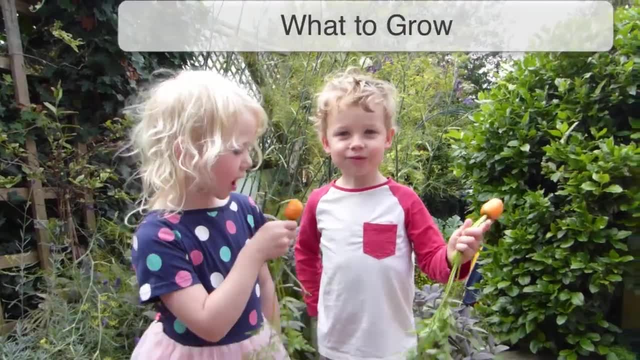 then have fun adding the plants. Clicking on the information buttons brings up growing tips along with suggestions for suitable companions to grow nearby. Children are far more likely to eat fruits and vegetables they've grown themselves- a great reason to get them involved in the process. 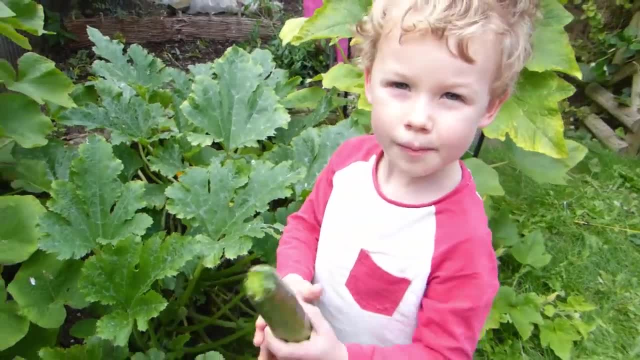 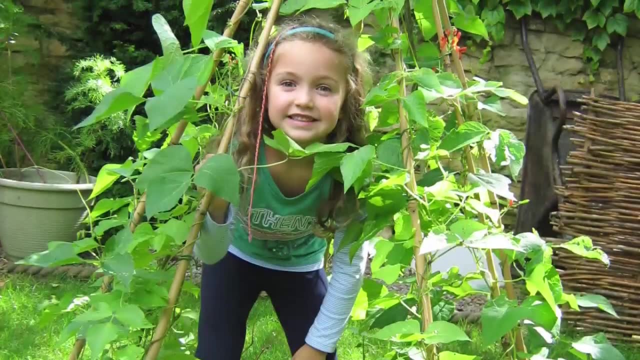 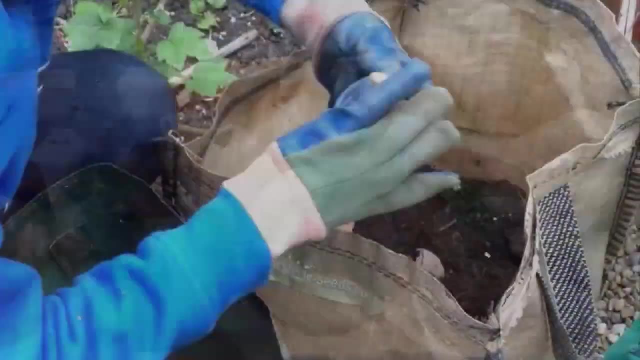 Choose crops that are robust, easy to grow and, crucially, ready to harvest during the term time. School garden staples include peas and beans. Children love sowing the fat seeds, setting up supports and, of course, picking the pods. Potatoes are fun to sprout before planting into potato sacks or beds. 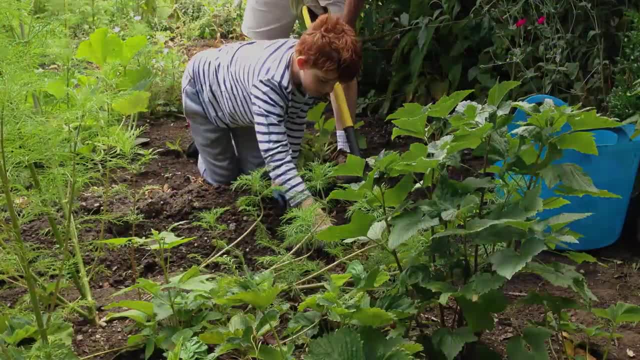 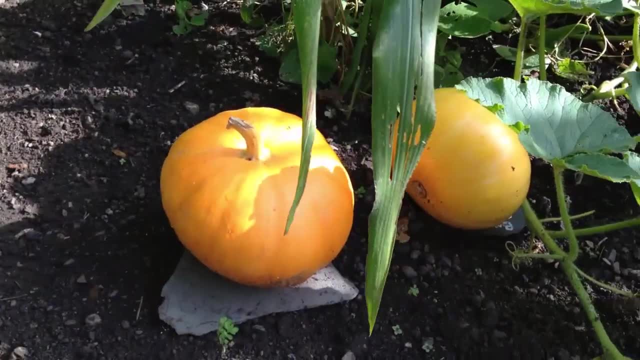 They'll love the hands-on growing process and unearthing the potatoes, nature's very own treasure hunt. Winter squash and pumpkins can be planted out at the end of spring and will be nearing maturity when the children return from their summer break. 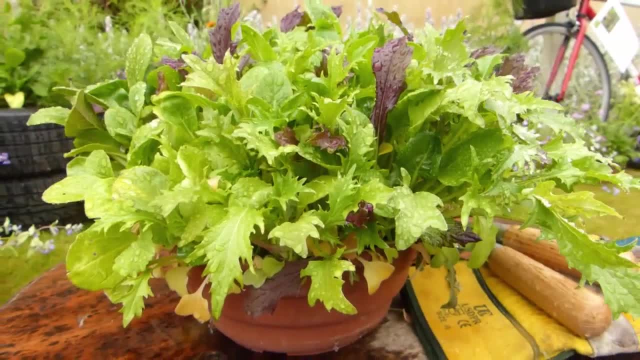 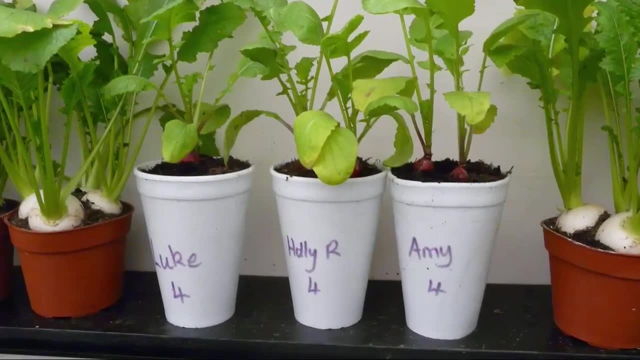 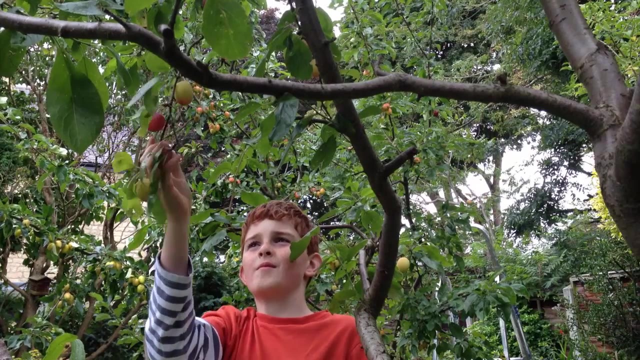 How about a pumpkin carving competition? Salads such as lettuce leaves and radishes are quick-growing and will keep youngsters engaged. They're also perfect for growing in pots to take home. Kid-friendly fruits include strawberries in raised beds and planters, plus all manner of fruit trees for an autumn harvest. 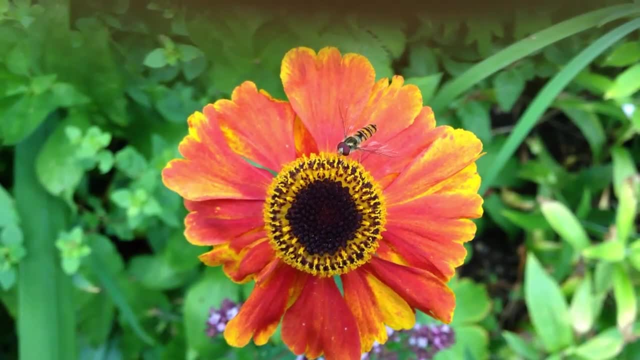 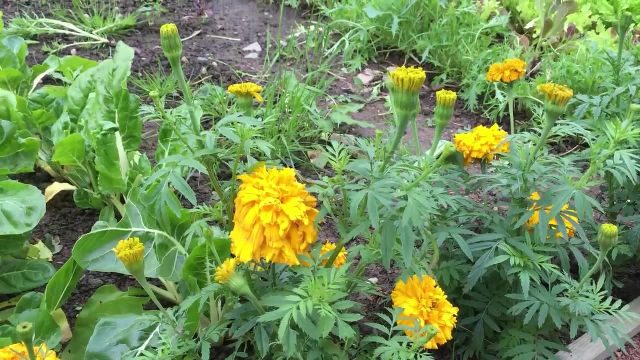 Flowers help to attract bees, butterflies and other wildlife into the garden. Children will love the splash of colour they give too. Annual flowers are quick-growing and should start blooming before the summer break. Think marigolds, nasturtiums, zinnias and more. 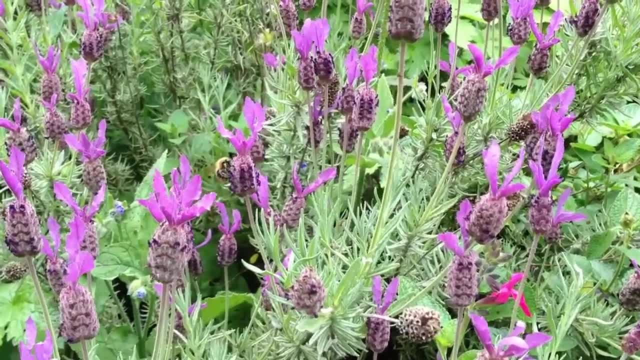 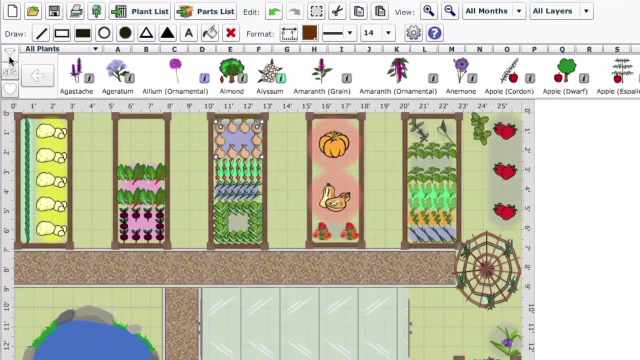 Don't forget herbs, many of which have beautiful bee-friendly flowers. The Garden Planner is a great way to start the summer. It's a great tool for choosing school garden-friendly plants. Simply click on the Custom Filter button, then select the Easy to Grow option to narrow down your selection. 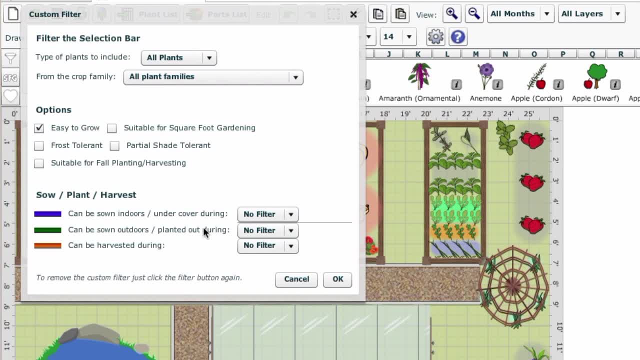 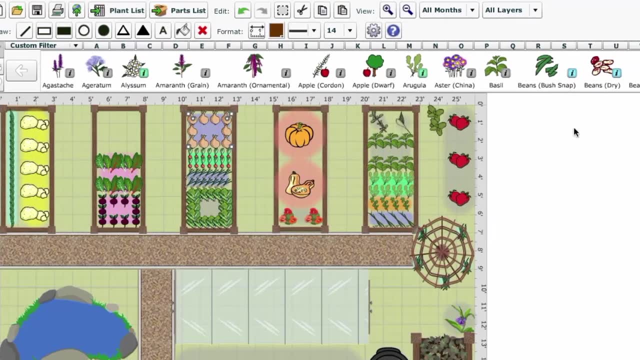 You can also use the Sow, Plant or Harvest filters to select crops that can be grown and harvested during the months the children will be at school. Click OK and the Plant Selection bar will be filtered accordingly, making decisions a lot simpler. 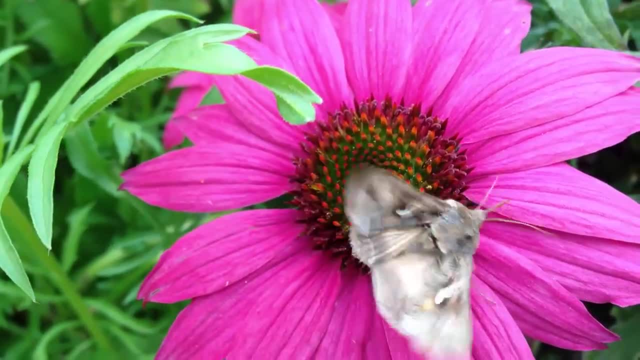 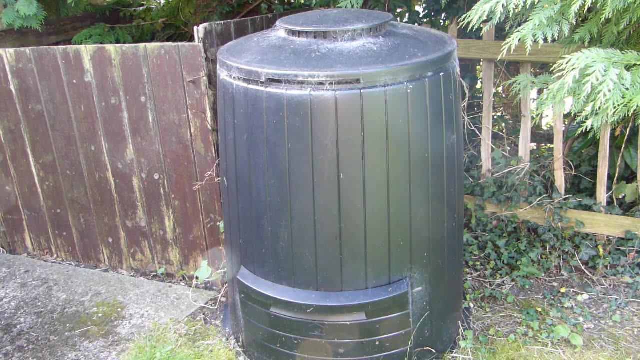 School gardens can teach children the importance of caring for the environment. School gardens can teach children the importance of caring for the environment and how nature works to feed us. Include a compost bin in your plan to show how old plants turn back into lovely. 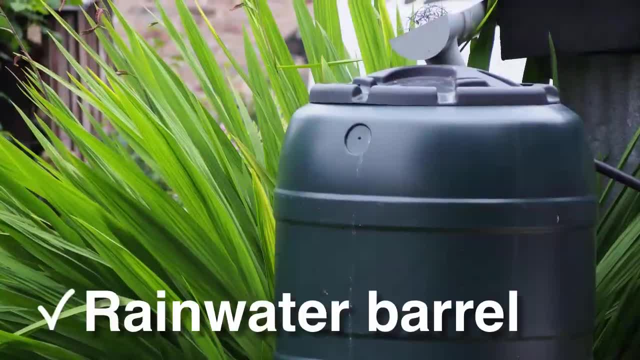 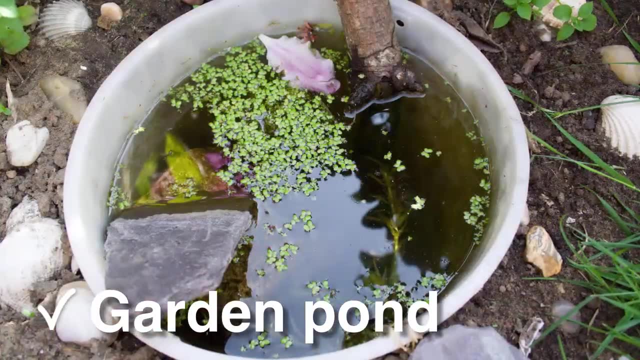 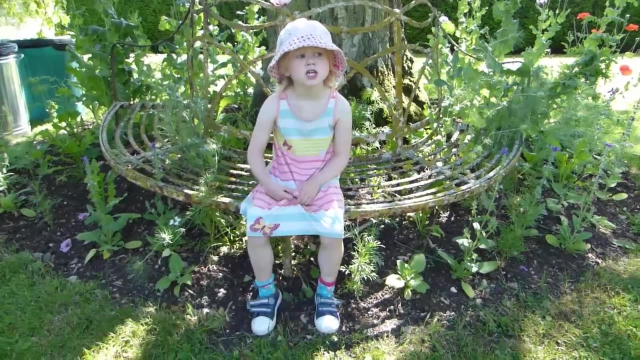 nutrient-rich organic matter to feed the soil. A rainwater barrel will demonstrate how to collect and make the most of precious water, while bug hotels and miniature ponds will draw even more wildlife in to study and admire. Make sure there's somewhere to sit during break times or outdoor lessons. 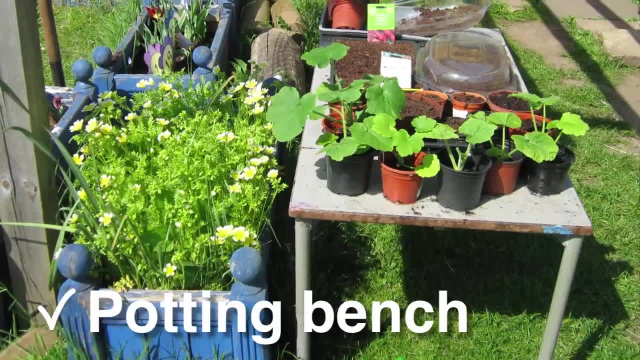 in the shade or sun, depending on your climate. Potting benches or tables are useful, but you can also use them to store food. Potting benches or tables are useful, but you can also use them to store food If you want to sow or plant up outside of the classroom. 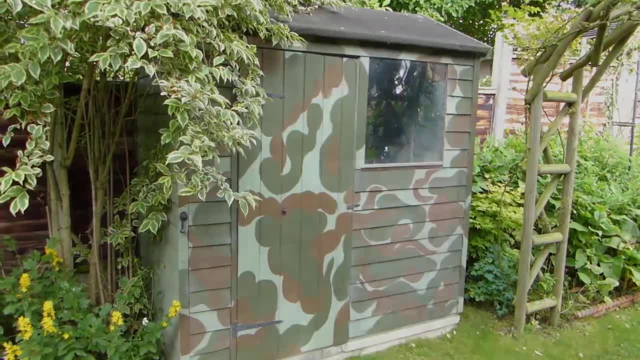 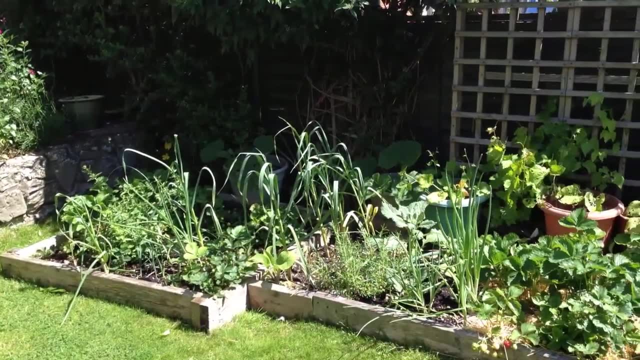 And, of course, you'll need a shed for storing your tools and equipment. School gardens are more complicated to look after than a home garden. Make it clear from the start who is responsible for what. Who will water the garden in dry weather? How will you order new seeds and potting soil? 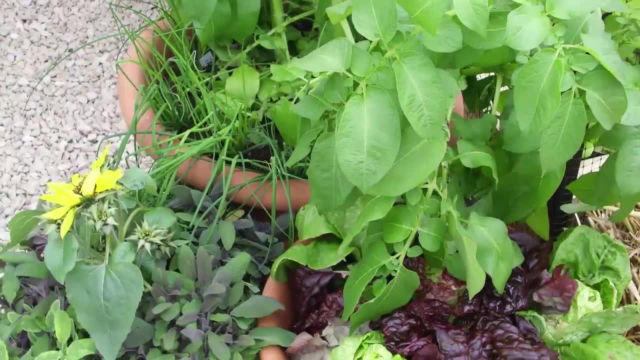 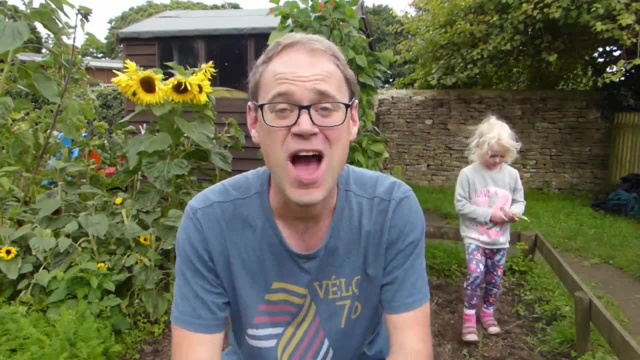 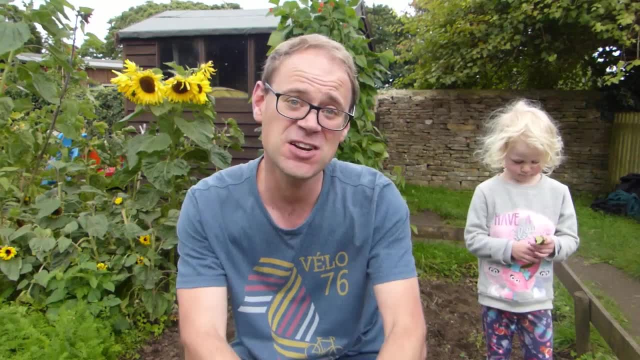 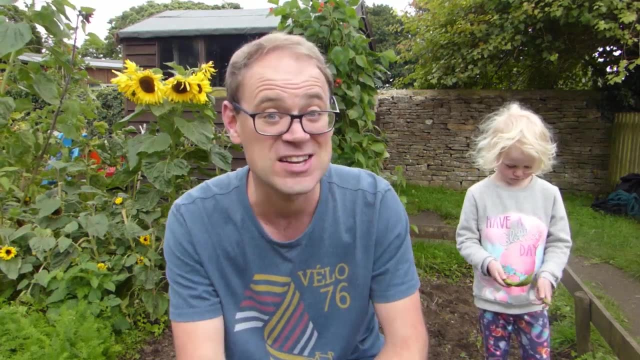 and a real love of wildlife and the great outdoors. Now, if you run a school garden, we'd love to hear from you. Please share your experiences and advice in the comments section below, And if you're not yet subscribed, make sure you do so before you head off. 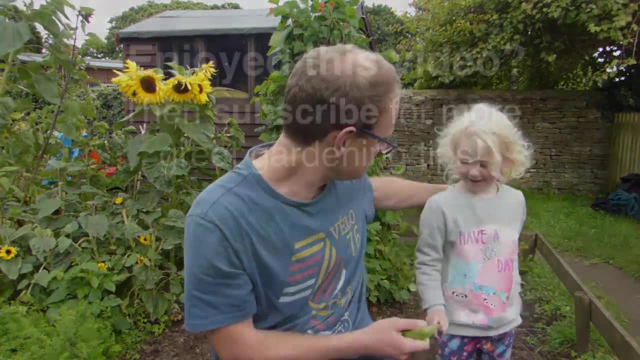 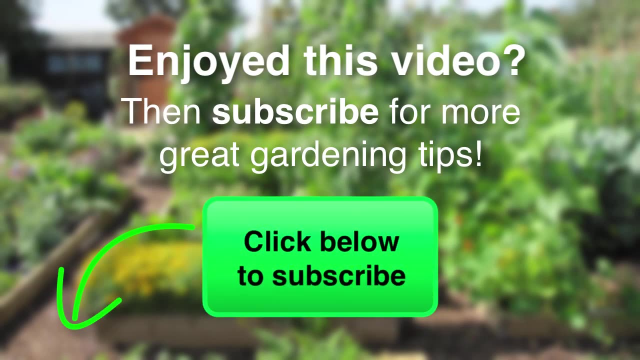 In the meantime, we'll catch you next time. Thanks for watching.